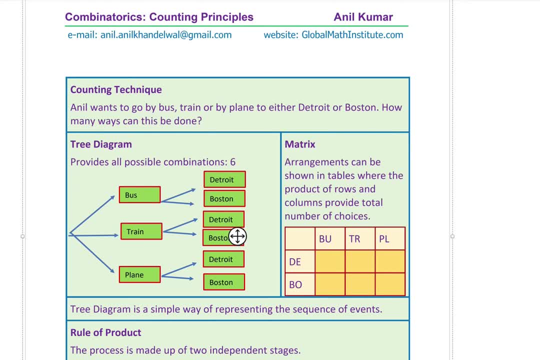 How many ways can this be done? So there are three ways of transport- bus, train and plane- and there are two destinations, Detroit and Boston. Now how many combinations do we have here? You could solve this question using a tree diagram, as shown here. 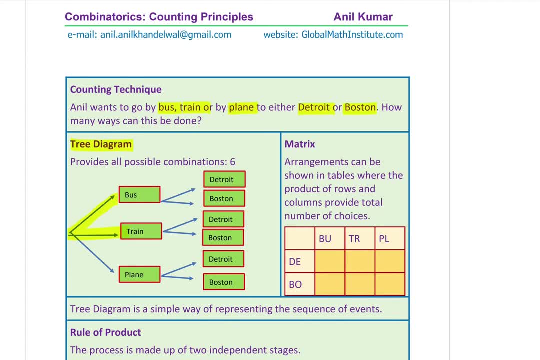 So there are three ways of transport. So these are the three options, and then the two cities, And that clearly gives you, in all, six options, right? So we have six ways of meeting this target. You could also do it with the help of a matrix, by drawing a table. 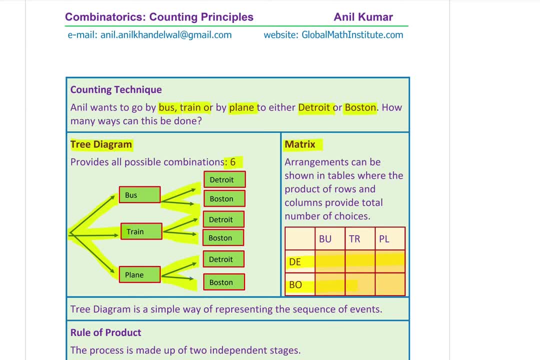 In this case, you could have two rows and three columns. Now, the two rows, which I have shown here, are the destinations Detroit and Boston, And the three columns are bus, train and plane. Well, that also gives you six cells or six choices. 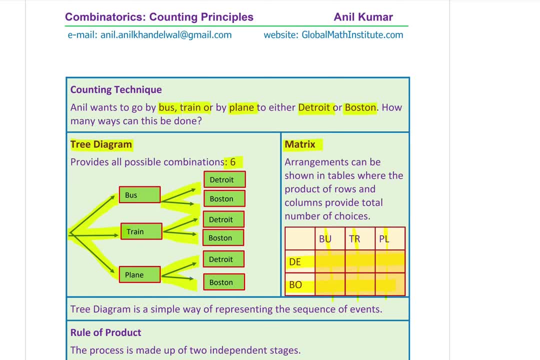 You get the idea Now. these techniques are very efficient if the data is very small, as in this particular example, And very conveniently we can figure out the choices. But there is a rule of product which we have seen here in both the cases: rows into columns. 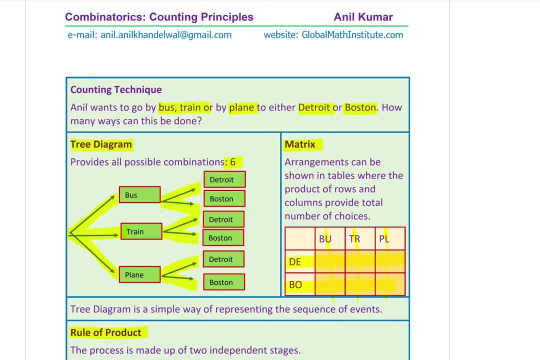 or the number of branches. Those here are the products. three into two, perfect, And that gives our first rule of counting right. So here you will notice that the process is made up of two independent stages. right, One stage is mode of communication. 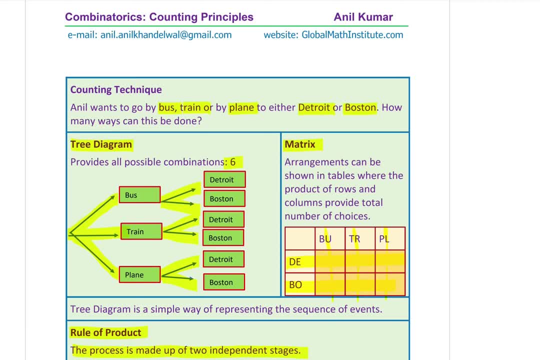 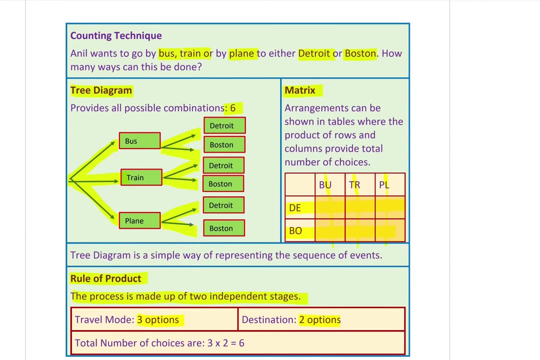 The other state is selection of the destination. So, mode of communication: three options. destination: two options for us. So, in all, what do we have? We have six options, correct? So, as you can see, here we have travel mode by two options. 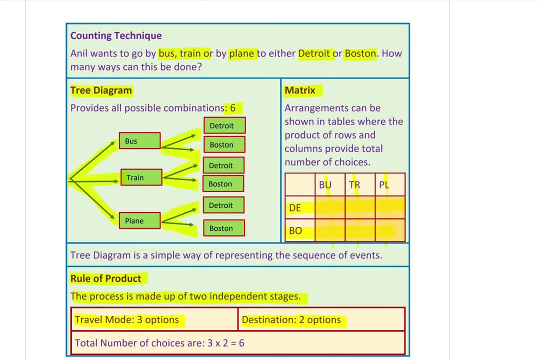 Destination is by two options. Travel mode is by three options- bus, train or plane. And destination- two options: Detroit or Boston. So the total number of choices are three times two, which is six, And this is called the rule of product. 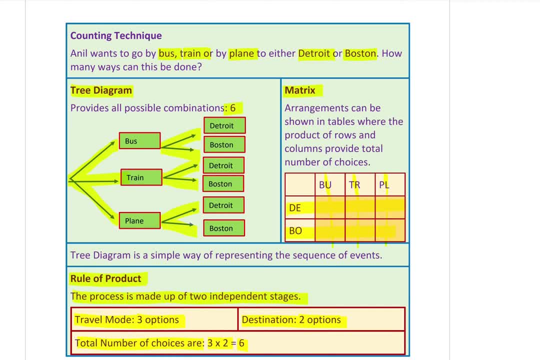 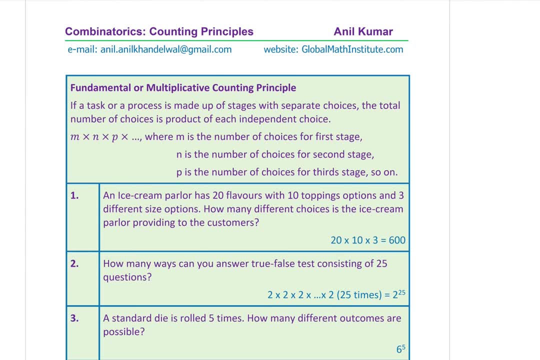 Okay, Now let's explore this rule of product. How can we use it very effectively? We'll follow up with some examples Now. we call this as a fundamental or multiplicative counting principle If a task or a process is made up of stages, as it was in this example, with separate choices. 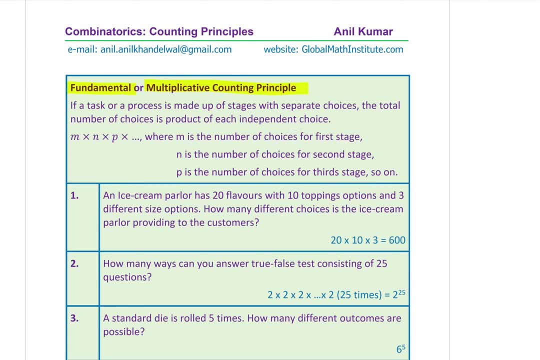 the total number of choices is the product of each independent choice. Correct, So, as in the last case, three times two. right. Three choices for mode of transport and two for the destination. So in that way we could actually extend it to any number of choices. 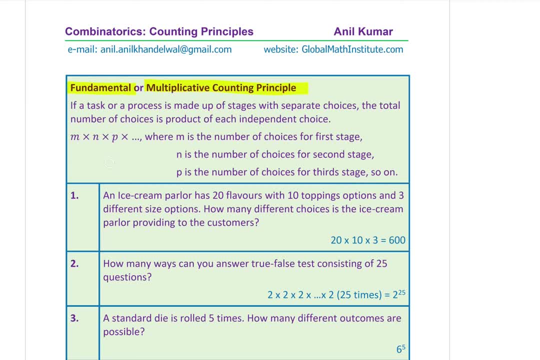 The condition is that they should be performed in a sequence right, And so, for choice one, if we have M options. for second, if it is N options and then P options, then the answer is product of all of them. Okay. 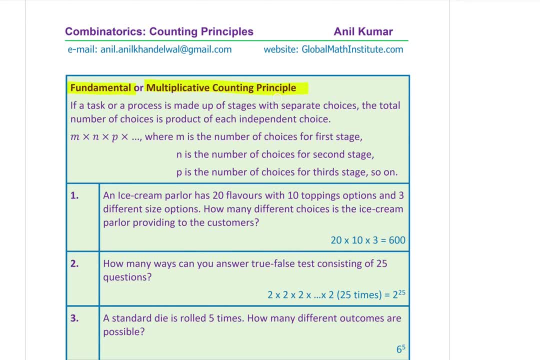 So that's what we call as fundamental, or the multiplicative counting principle. Okay, Let's take a few examples to understand it. Example number one: here is an ice cream parlor has 20 flavors with 10 toppings option and three different size options. 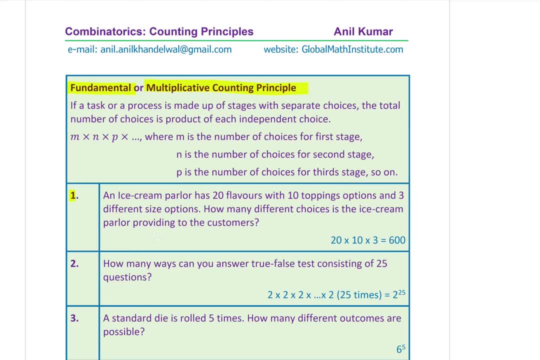 How many different choices is the ice cream parlor providing to the customers? Well, there are 20 flavors independently, right Times, 10 toppings, Okay- And three serving sizes. So we can just multiply the three and get the total as 600 in this case. 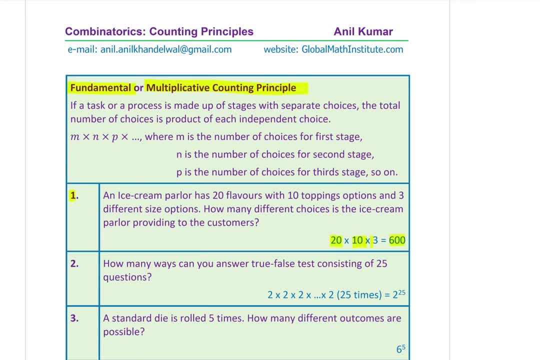 How simple it is correct. So if you identify that there are three independent ways which could be done in a sequence and operation, you understand, in that case just multiply them and get the answer. Let's take another example, example two: how many ways can you answer true or false test? 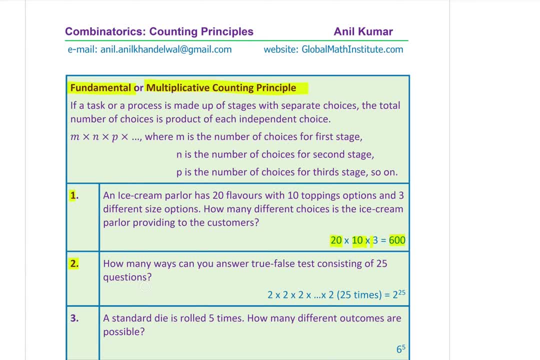 consisting of 25 questions, So we could say true or false. that means we have two options right For every question. we have 25 questions. two times two times two times two, So two to the power of 25, will become the answer. 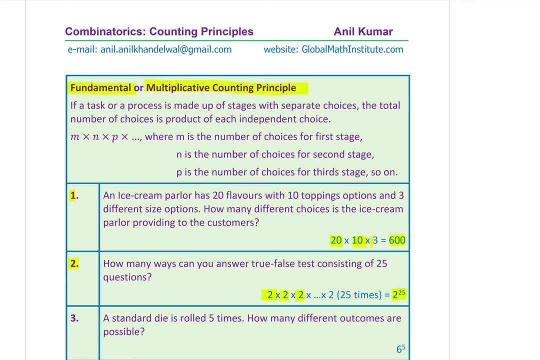 So keep on multiplying by two every time, right? There are 25 questions, so every two gets multiplied and we get two to the power of 25 as the answer of this question. Okay, Now let's look into question number three, which is a standard die is rolled five times. 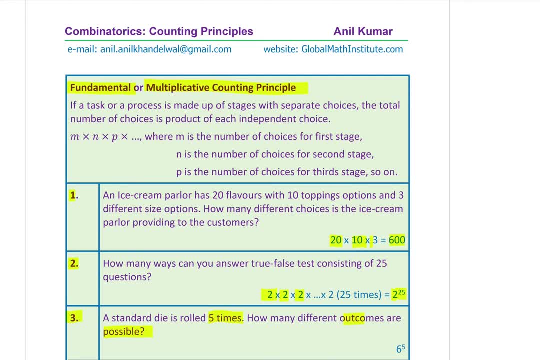 How many different outcomes are possible. So we have used a technical word, outcome, here, which will be very popularly used when we talk about probabilities, right? So number of outcomes means what results come out of a single throw of the dice. So when you throw a die, you get six options, correct? 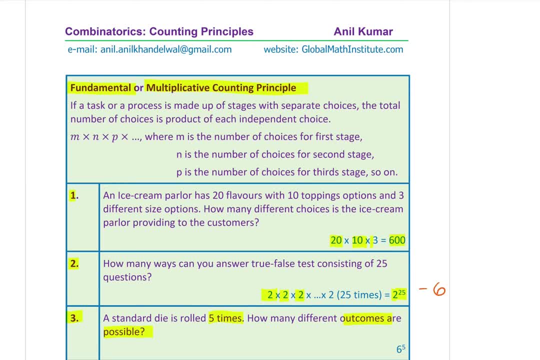 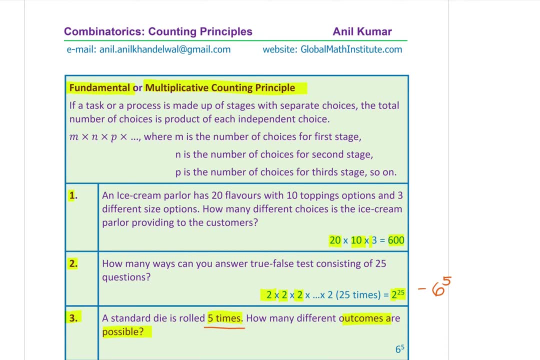 So every time you throw a die, you get six options correct. So every time you throw, we get six options right. So if I do it five times, then it will be six to the power of five as our answer perfect. 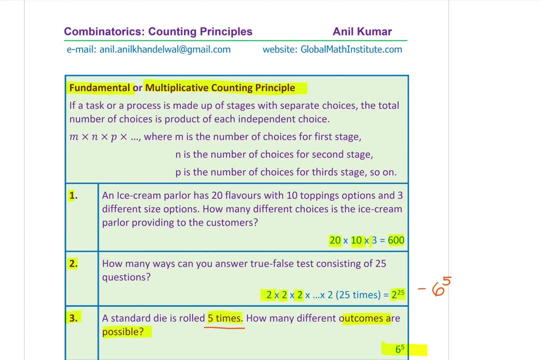 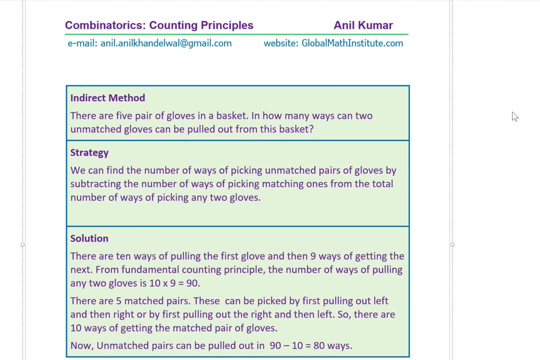 So that is how we could apply this rule of multiplication and get quick answers to some questions. Now let's look into another method of doing these things. Sometimes we also follow indirect method of counting. Now let's look into this indirect method, Indirect method of counting. 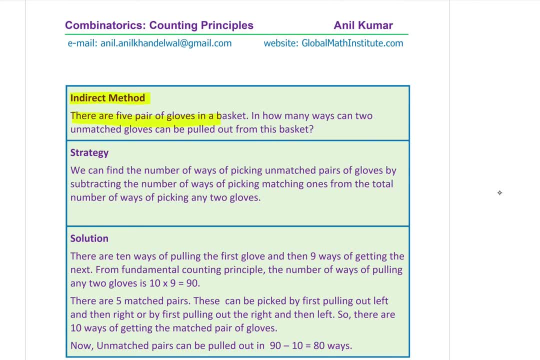 Example here is: there are five pair of gloves in a basket. In how many ways can two unmatched gloves can be pulled out from this basket? So in this case we are pulling out and we are interested in finding unmatched gloves. right Now there could be many options to get unmatched gloves. 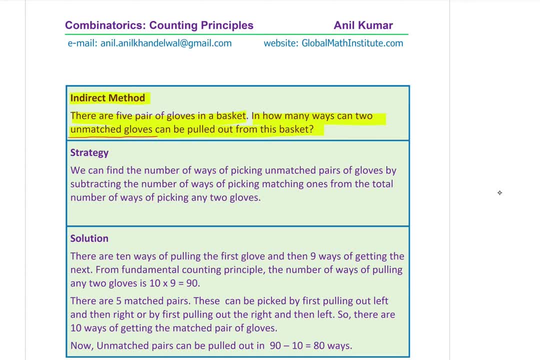 When we say indirect, we say: well, what we could do here is we could say: well, let's do this, We could find total options right And from them we could deduct matched options, And that will give us the options for unmatched. 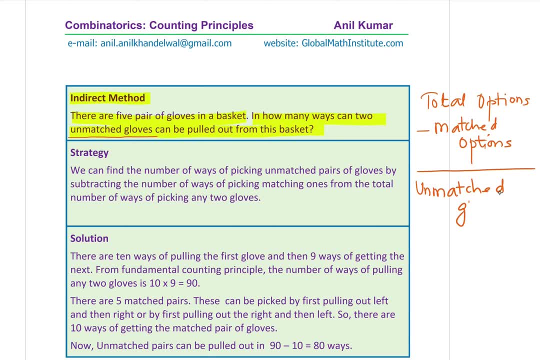 Does it make sense? So that is what we are calling as indirect Perfect. So we could do it like this, So that is our strategy. So the strategy here is that we can find the number of ways of picking unmatched pairs of gloves by subtracting the number of ways of picking the matching ones from the total. 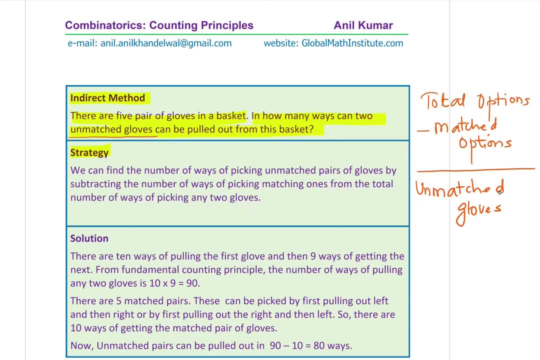 number of ways of picking any two gloves- Perfect. Now let's see how to solve it. So there are 10 ways of pulling first glove And then nine ways of getting the next. So what we're trying to say here is: let's say, there are 10 gloves, right? 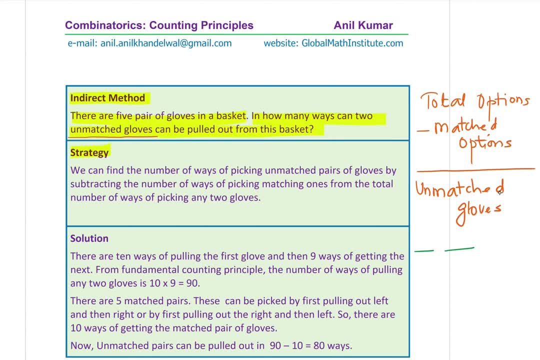 So we have to just pick two. So we have the option whenever we try to pick it. for the first time, we could pick any one of those 10.. And the second time, since one has been picked, we have nine left there. 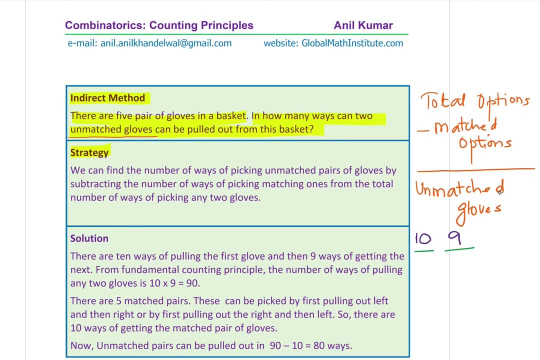 So there is option to take nine. now, right, So there are 10 ways of pulling the first glove. Okay, So there are 10 ways of pulling the first glove and then nine ways of getting the next. since we have picked one From fundamental counting principles, the number of ways of pulling the two gloves is: 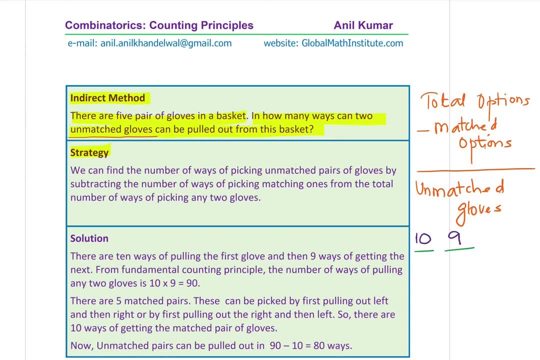 10 times nine, which is 90,. right, So we get the total options of pulling this pair. So there are 90 ways of pulling the pairs. Now there are five matched pairs, right? Okay, Now, when you have five matched pairs, then these can be picked by first pulling out left. 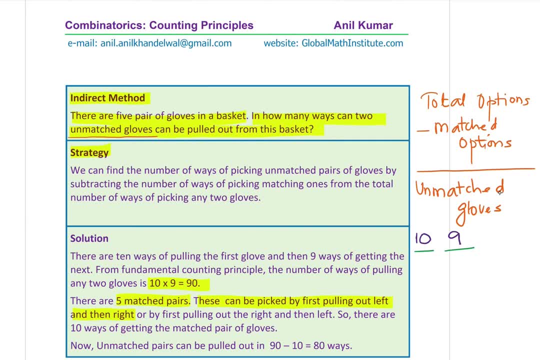 and then right, okay, or by first pulling out the right and then left. So both ways you could match up here. So there are 10 ways of getting the matched pair gloves right. So first five are the correct ones of the left side. 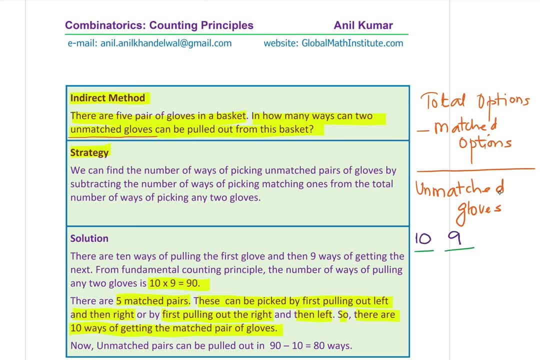 And then you pick up: Okay, From the right side, right. So that is how we have 10 options, 10 ways of getting a matched gloves, And unmatched will now be difference of total with the matched ones, And we get 80 ways as our answer. 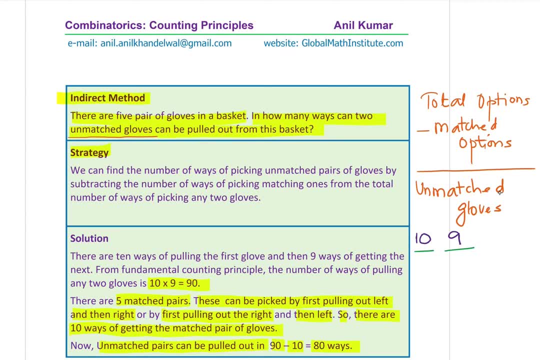 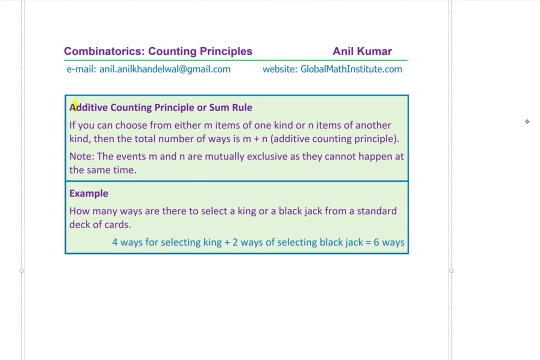 So that is what we calling as indirect method- Perfect. So it is easier in this case to figure out how many options are there for pulling out matched pairs. We found our answers indirectly and it is a very efficient way of working. Now let us look into the second principle, which we call as additive counting principle. 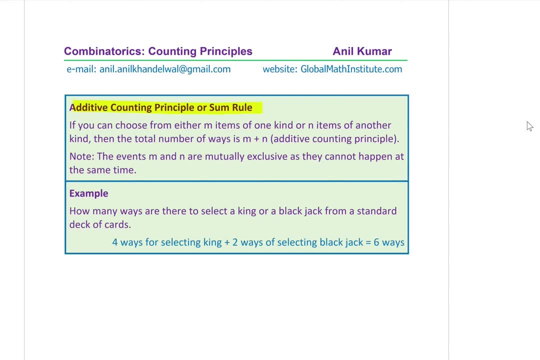 or the sum rule, If you can choose from either M items of one kind or N items of another kind. So there are two types of items, right? Mutually exclusive. we say There is nothing overlapping here, right? So if you can choose from either M items of one kind or N items of another kind, then 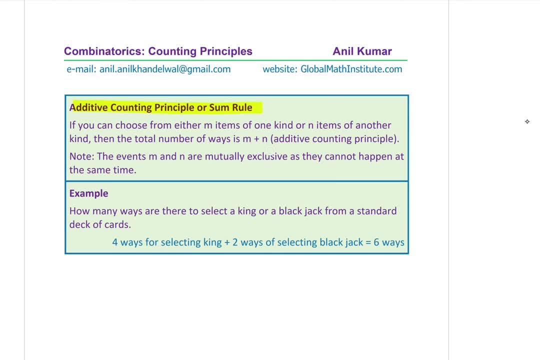 the total number of ways is M plus N. Additive counting principle: right. That is what we call as additive. And this is like we have OR operation going on, correct. So either this or that, That is what we call additive. 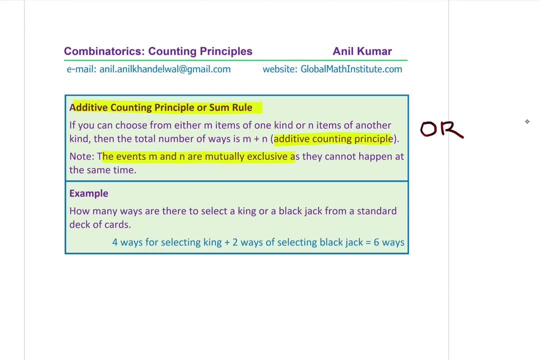 Note: The events M and N are mutually exclusive as they cannot happen at the same time. right, This is very important. So the two events should not be overlapping, They should be mutually exclusive. Nothing common between the two. Example here is: how many ways are there to select a king or a black jack from a standard? 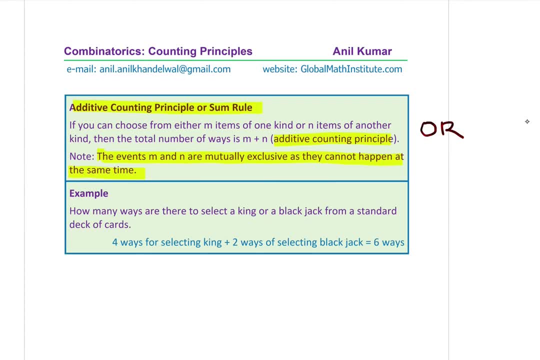 deck of cards. Well, If you select a king, you cannot select a black jack, correct? So there is nothing overlapping. So these type of events are called mutually exclusive. right Now, as you know, in a deck of cards we have 52 cards, correct? 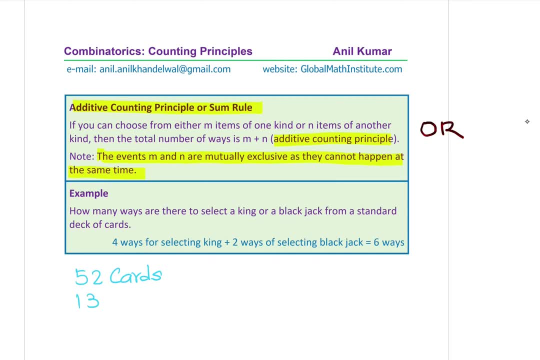 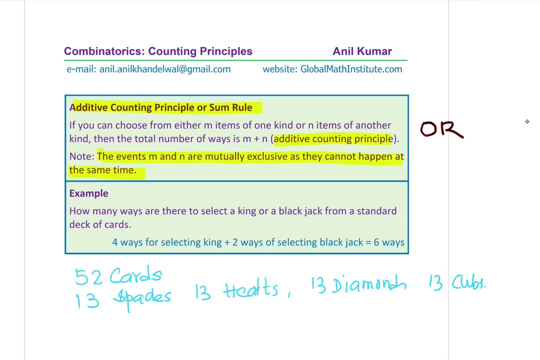 These are called suits. So there are four suits, Each 13,. right, We know that 26 are red cards And we know that 26 are black cards. the numbers go from 1 to 10, and then we have Jack, Queen and King. one is like ace. 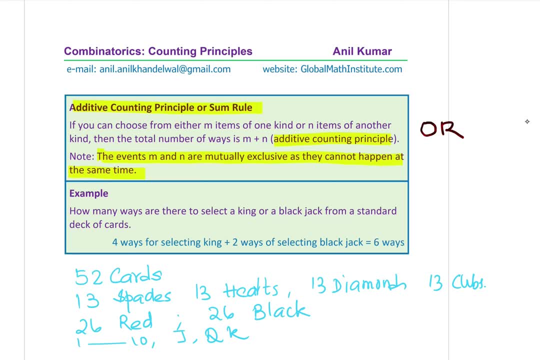 right? so these are the 13 cards which you are playing with. so now, in this particular case, as you can see, we have four Kings, correct? so there are only four ways of selecting a king. now we're talking about blackjack. there are four jacks, out of which two are black jacks, two are the red jacks, correct? so the red 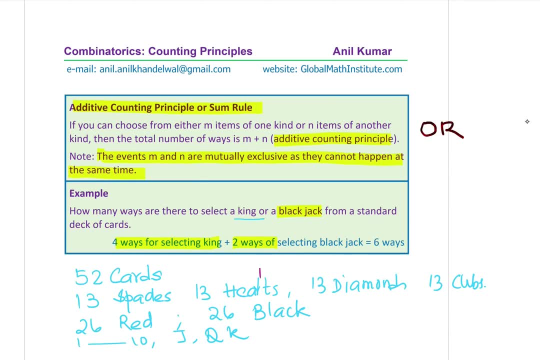 ones are the hearts and diamonds, these are red, so and the black ones are club and spades. so when we are saying two ways of selecting backjack, that means there are only two cards. so we have in all six ways of getting either one of those Kings or 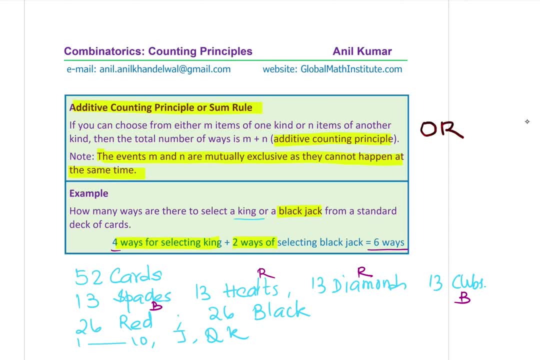 one of those black jacks, right? so how many ways are there to select a king or a blackjack? either one of these two, right? since there are only four Kings, those are the four ways, and since there are only two black jacks, there are two ways. so in all, we have six ways of selecting a king or a blackjack card. 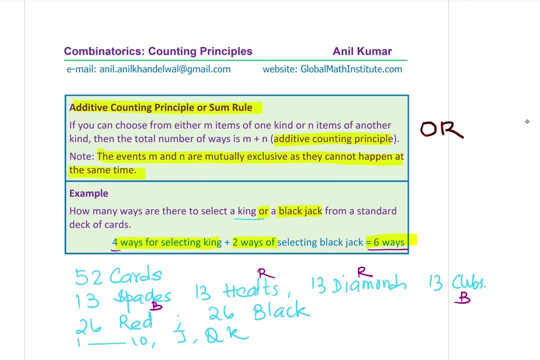 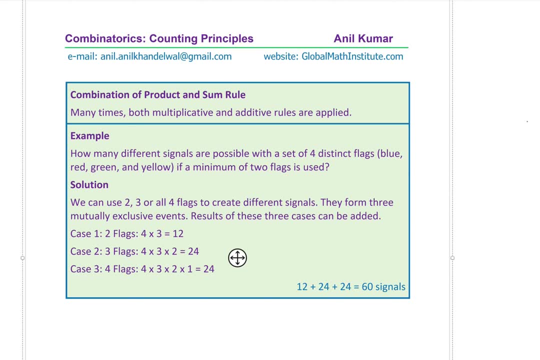 keyword is: or here. in that case you can add: right. let's take few examples now based on this. so here we'll talk about combination of both product and some- as that may be the case in many times, so many times- both multiplicative and additive rules are. 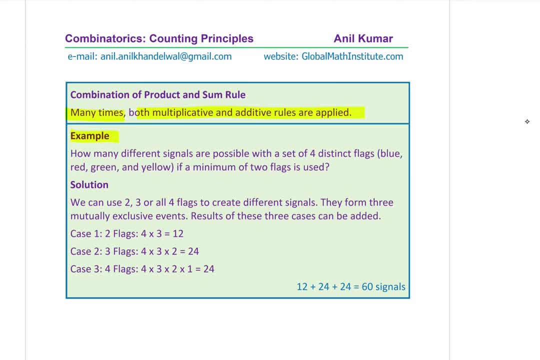 applied? here is an example: how many different signals are possible with a set of four distinct flags? let's say we have four flags. their colors are blue, red, green and yellow. so they are very different flags, different colors, if a minimum of two flags is used. so the question is: how many different signals? 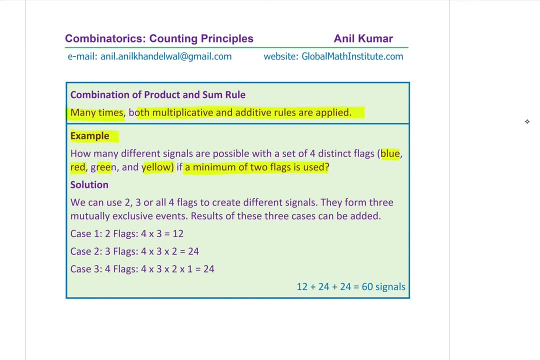 are possible with a set of four distinct flags if a minimum of two flags is used. now, when we say minimum of two flags is used, that means that you could use two flags, you could use three or all four, right? so these are the three cases. we call them as cases, so we have to work them separately. 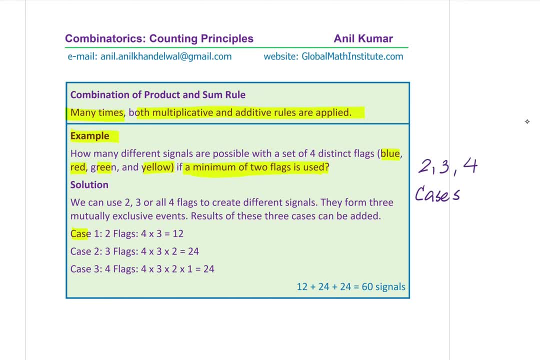 so we have accordingly define our cases: case one using two flags, case two, when three flags are used. and case three when four flags are used. right, so we can use two, three or four flags to create different signals. their combinations will give different meanings. right, they form three mutually exclusive events. 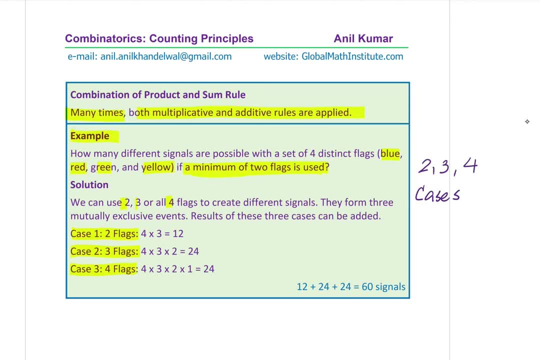 results of these three cases can be added. you understand? so if you are using two, you are not using three flags, right? so they are mutually exclusive. now let us say that you are using only two flags. that means we can think about two positions to be filled, since you are using two flags. but we have how many we? 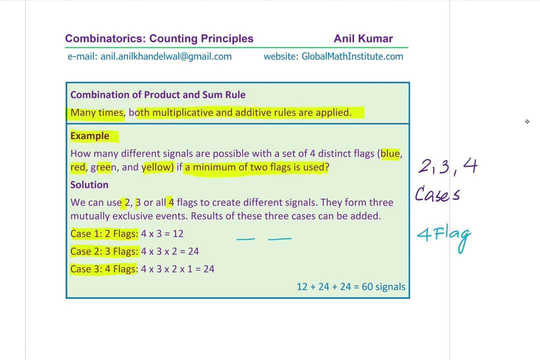 have four flags in all, correct? well, we are using two for signaling. in that case, you have a choice of four. but once we pick up one of them, in that case three are left, so we get four times four. in that case, three are left, so we get four. 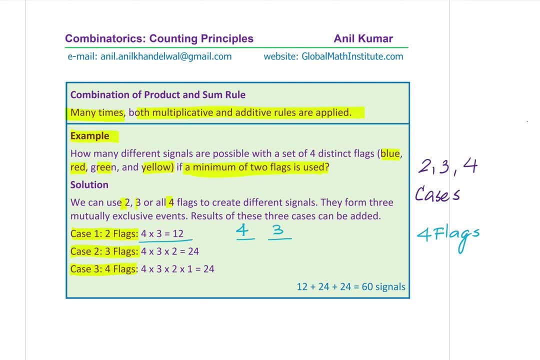 times three, as twelve, as a number of choices when two flags are being used. well, if you're using three flags, in that case to pick up the first we have four. then, once we have picked up a flag, three are left, and if that has been also picked, 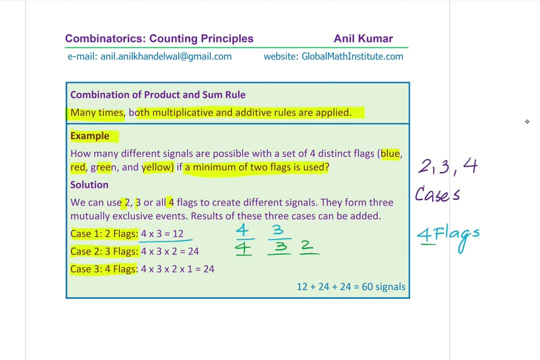 then we have a choice from two. so the total is four times three times two, which is twenty-four. now, if you have to use all the four flags, which is also an option, in that case, first you have a choice for four, then three, then two and then one. so we have a choice of 24 options, when all the four 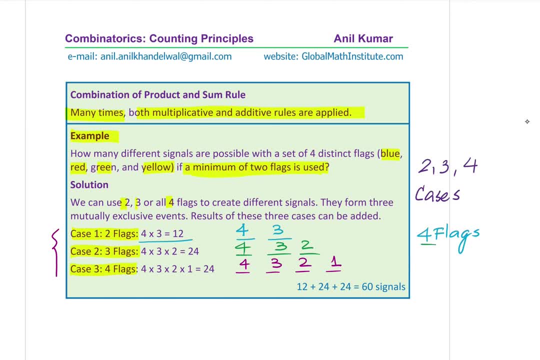 flags are used. now, total is all the three cases together. since the question says that a minimum of two flags is used, that means two flags could be used, three flags could be used or four flags could be used- perfect. so we can add them all to get our answer, which is 60 signals. so we can provide 60 signals by 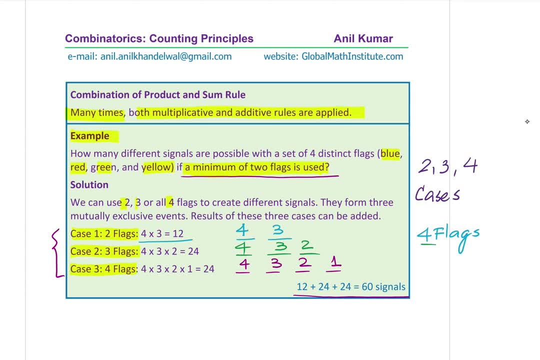 using four flags and at least two of them together. perfect. so that is all. as you can see, here, we have used both the principles, the multiplicative, for individual options, and then, since the events are mutually exclusive, we added the results. now let's take some more examples now. here is a practice. 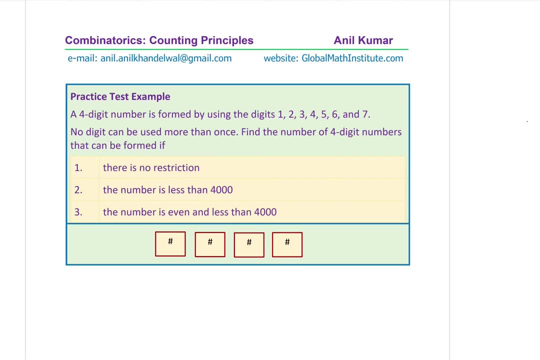 test question example. The question is right before you. I'd like you to pause the video, answer the question and then look into my citations. A four digit number is formed by using the digits 1,, 2,, 3,, 4,, 5, 6, 7.. So there are seven numbers. 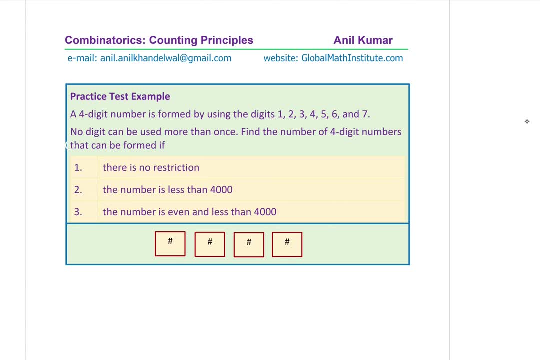 and we are only choosing four of them. No digit can be used more than once. Find the number of four digit numbers that can be formed if there are three cases. First, there is no restriction. So if there is no restriction, then how many? 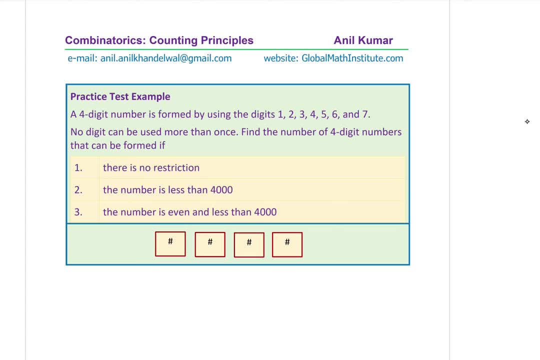 four digit numbers can be formed using the numbers 1,, 2,, 3,, 4,, 5,, 6 and 7.. That becomes the question. Question number two: here is the number less than 4,000.. So you. 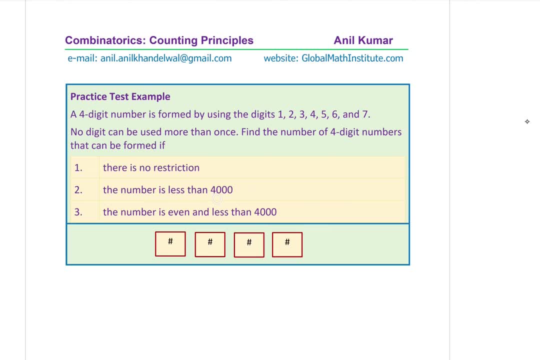 have to form a four digit number which is less than 4,000, using the digits 1,, 2,, 7.. And third option is that the number is even and less than 4,000. Perfect. We'll use our rules of multiplication or addition to find the answer right, So I. 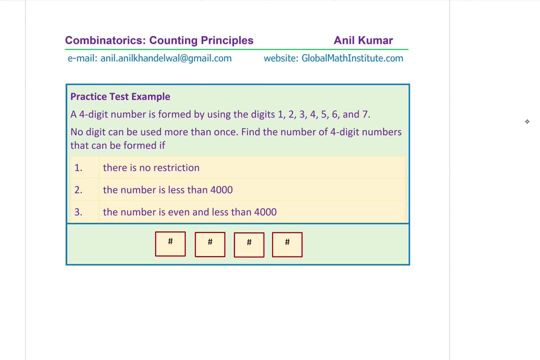 have made four boxes here. Think about choosing a number in each box, correct? So that will give you a four digit number. So now, if you look into the first case, which is there is no restriction, we have to make four digit number using these. 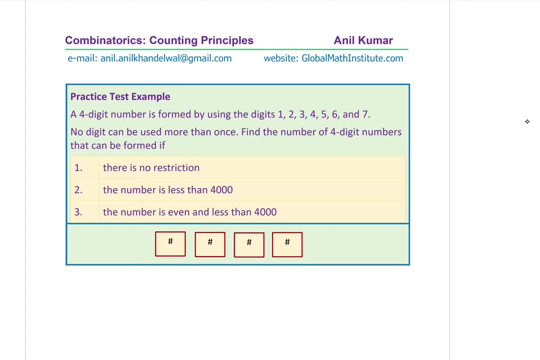 seven numbers. In that case, in the first box I have a choice of seven numbers, correct? So I can choose seven numbers for one box. Once I do that, then I'm left with six numbers. So I can choose from those six numbers When I pick up the two. 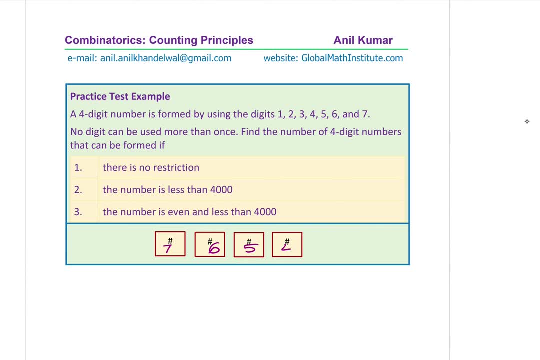 I'm left with five, and then I'm only left with four. So the total number of choices for the first case, when there is no restriction, is seven times six times five times 4.. Is that correct? So that is how we could easily answer the question using. 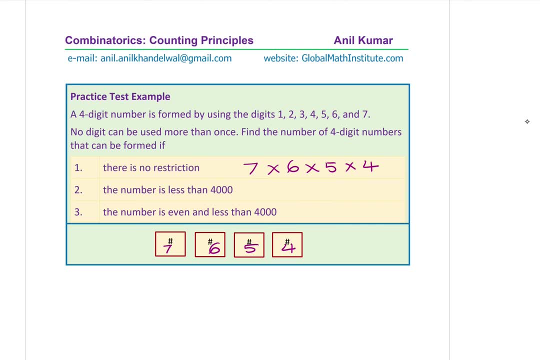 our first fundamental rule of multiplication. Since these are independent events, right, So first box, we could choose 7.. Once it has been chosen, then we are left with 6 numbers to choose from, and that is how we get our answer. So now I'd like you to answer question number 2 and question number 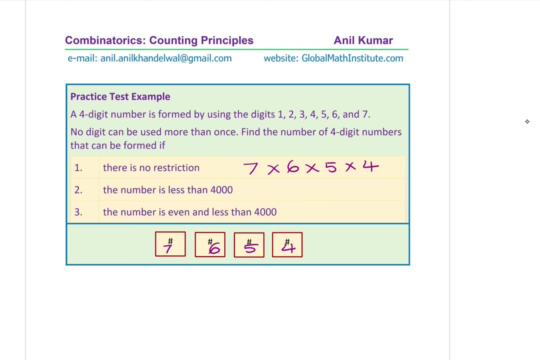 3 on this information. Okay, so I hope you got the answer. Now let's look into how do we work with it. Number: less than 4000.. When I say that the number is less than 4000, that means the choice is restricted. I can only use 1,, 2 and 3 for. 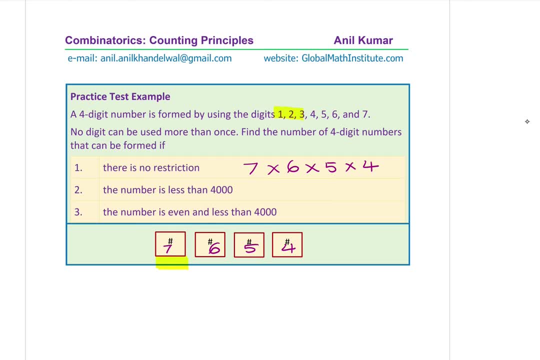 the thousand players right. So at this place, I can now choose only one of these three. So therefore, here I have only three options left, So I can now choose one of these three. So therefore, here I have only three options left. Now, if I choose one of these three for the thousand players, in that case I am. 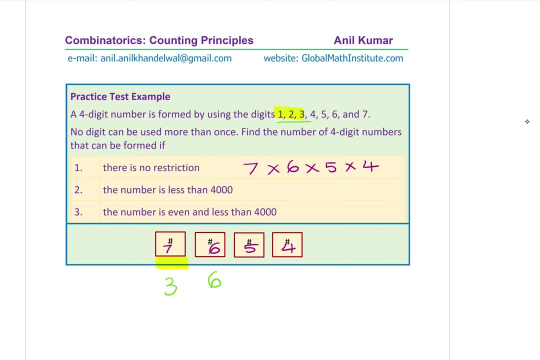 left with six options, and there is no restriction to that. Any six of those could be now chosen. The number is going to be less than 4000, for sure, and then five, and then four. So in this case, the choices will be three times, six times. 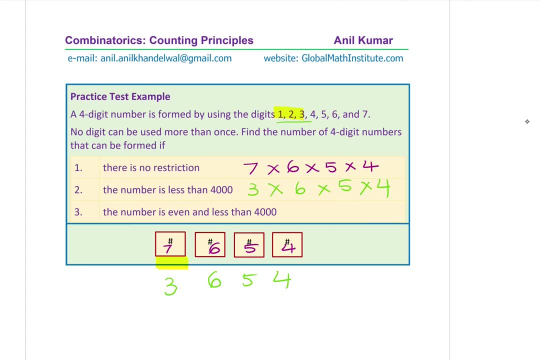 five times four. You can always multiply them and get your answer, Of course. Now the question here is: the number is even and less than 4000, right? So I like you to think about it. Even means what? Even means that the last. 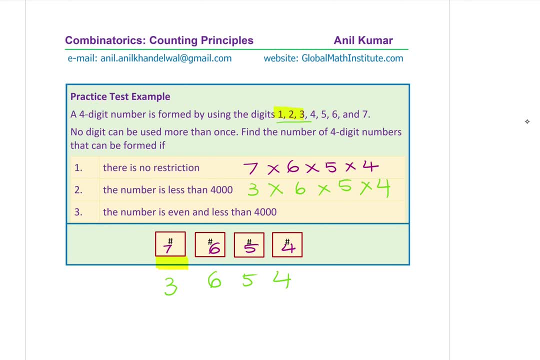 digit is now restricted. We could only have two, four or six in the last place right. And also we have a restriction that in the first place we could only have one, two and three. Now we have got two types of restrictions. One is that the number is less than 4000. 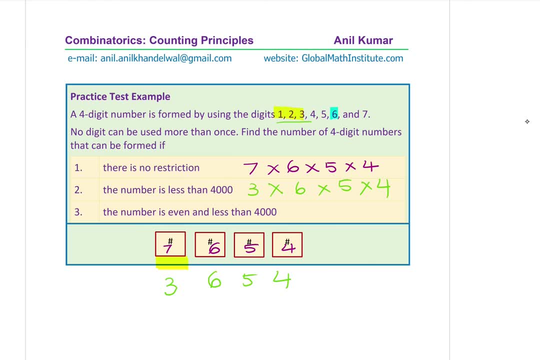 The last digit could be only six, four or two. You can clearly see that if two is in the last place, in that case, in the first place, we are restricted with only two numbers: one and three. You get the idea. So those are different cases to work on. 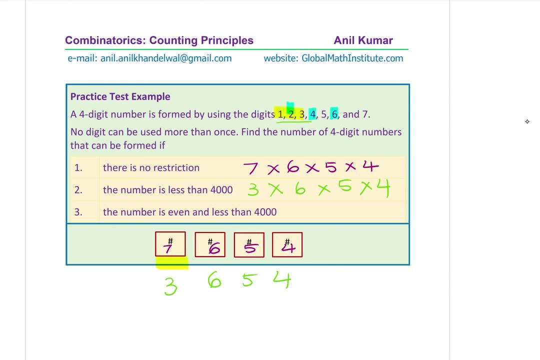 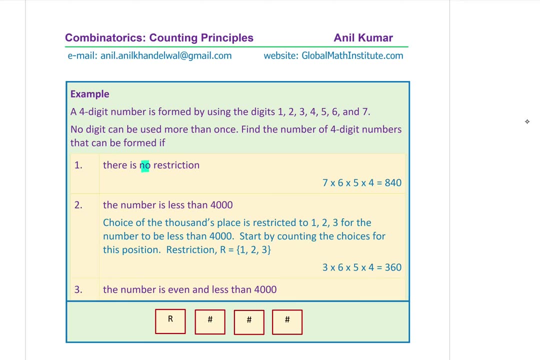 So I like you to focus on this and then look into my suggestions. Okay, let's move on and see the results. Well, the first case was very clear: No restrictions at all, and you found it will be seven times six times, five times four getting the answer of 840. 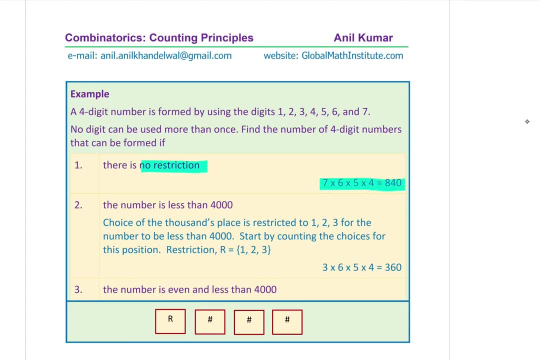 no restrictions. now, in the second case also, we saw that we ordered a number which is less than four thousand. so first position was restricted to three choices: one, two or three- and then six, five and four were the choices and the results into 360 choices. now we're trying to figure out. 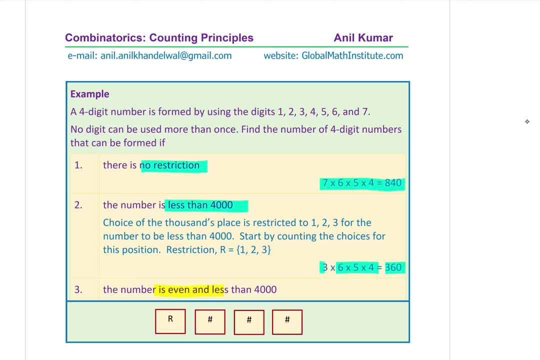 the number of ways that the number is even and less than four thousand. so clearly, the choices for the first digit are one, two and three, and the choices for the last digit are two, four and six. now, based on this, we have to work out the details right. so we have three different. 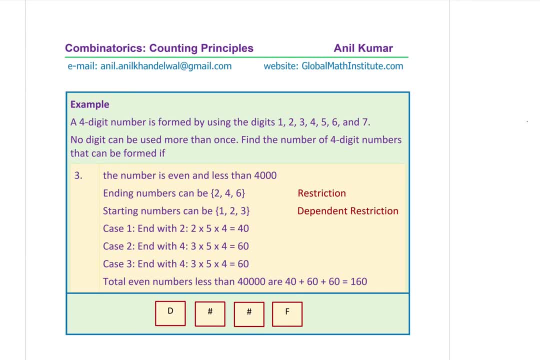 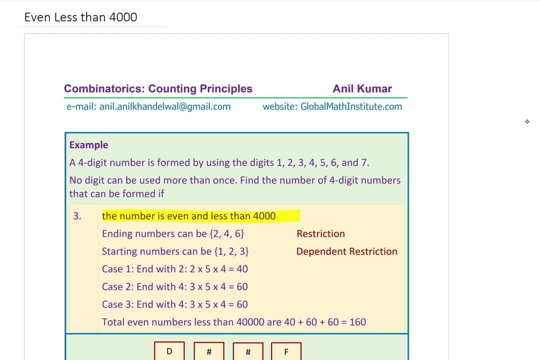 cases to work with. now let's look into these cases one by one, correct? so now the number is even and less than four thousand. right, that is what we are now looking into. so let's see: the number is even and less than four thousand. that means the ending numbers are two, four and six, and 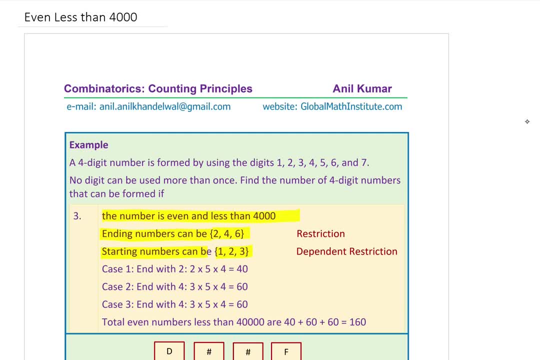 the starting numbers are one, two and three. now important thing here is to understand what is our main restriction, even numbers. well, let's take that as a main restriction. so that means we'll first fill up the ones place, right? so one's place could only take these three items, so we'll start with the ones place. that is our. 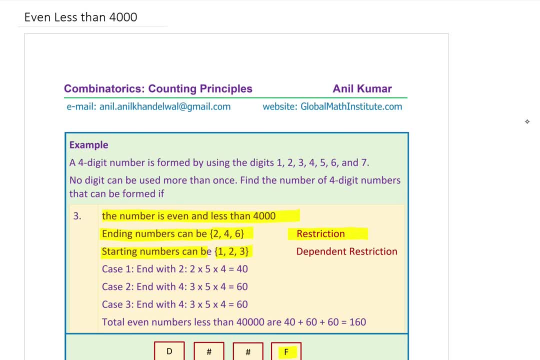 that is fixed now, once we have fixed that, in that case, dependent restriction is that the starting position cannot have the number which has been fixed, right, so that call- let's call this as a dependent number. well, once this number is fixed, let's call this as a dependent number, well, once. 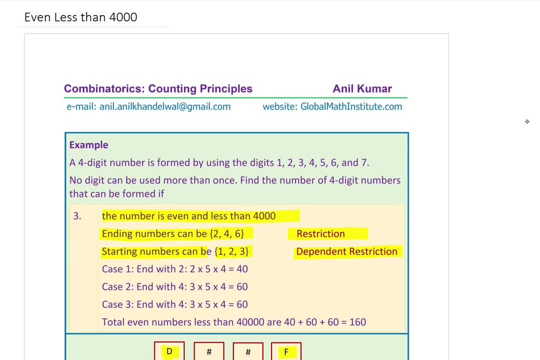 these two are filled in, then in between there is no difficulty. we will fill in the remaining, correct. so one and two are gone, so all of seven. two are gone in the first and the last case. so we are left with how many? five and four. so they will take the next two places, correct, of course. 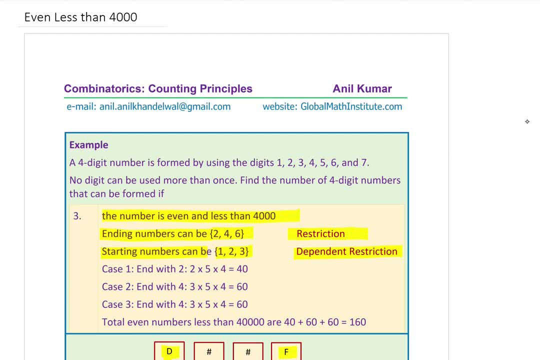 now let's see each case one by one. so let's work out the first case, which is case one where the number is ending with. Now, if the number is ending with 2, let me write down a number ending with 2 here, right? 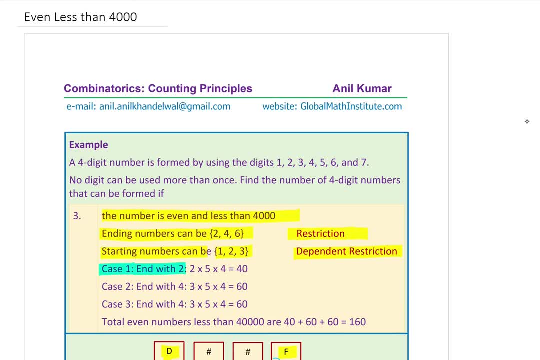 So let's write down 2 ending number here, okay? So if number is ending in 2, then in the first place I cannot write 2.. I have only choice for 1 and 3, do you see? So that means when number is ending with 2, I have a choice of only placing two numbers. 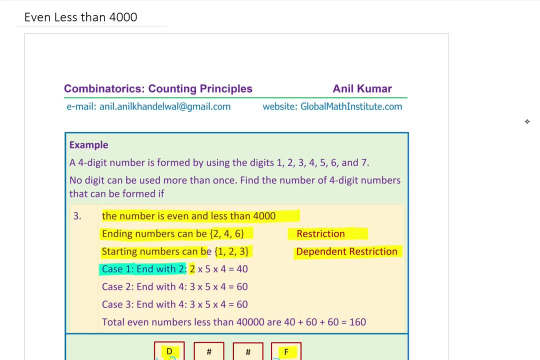 in the first position, correct? So I have utilized 2 numbers out of 7,. 5 are left. that is placed here and then 4 left goes to the next position. So when I place 2 in my final position, in that case there are 40 ways of filling this. 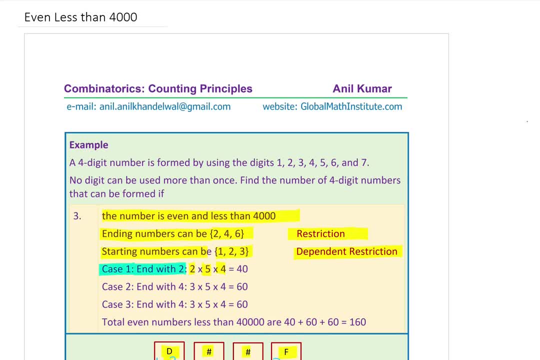 up right. Now let's look into the case 2.. Now case 2 is ending with 4.. Now if I write 4 over here as the last option, In that case I have all the 3 numbers- 1, 2, and 3, which can be placed here in D right. 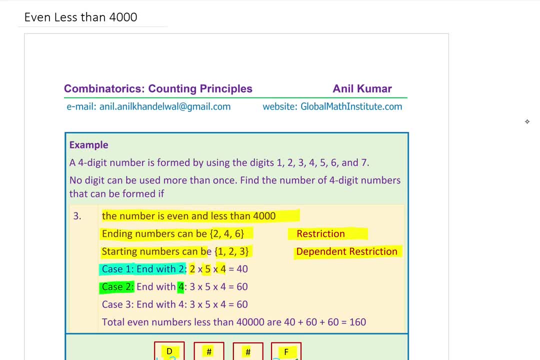 Do you see that? And therefore, as you can see clearly, we have 3 options And for those, 2,, of course, 5 and 4, which is common, right? We have placed 2 numbers, we are left with 5, and then 4.. 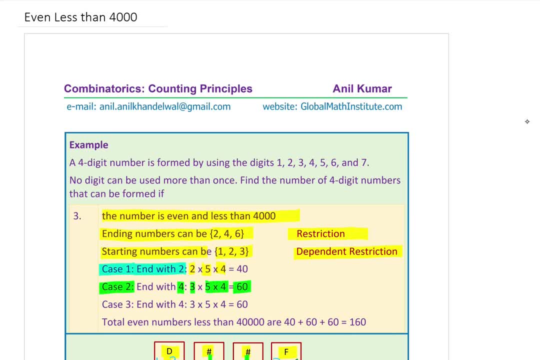 So we get total of 60 options. Similarly, if I choose 6 as my last number, in that case again I have 3 options for the first one, Which are 1,, 2, and 3, correct. So again I've got 3 times 5 times 4, and same result as 60 as the last time. 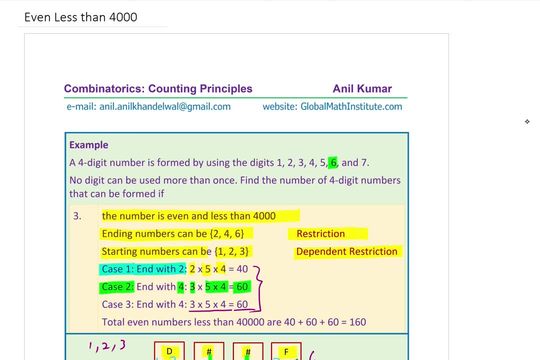 Now, in the 3 cases which you're talking about, we can add them up to get the total number of ways of having even numbers less than 4000.. So that is 160, 40 plus 60 plus 60.. Is that clear to you? 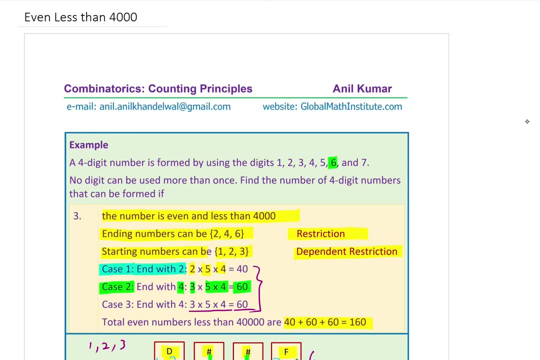 So, when we are talking about the combination of 4 and 4. When we are talking about the counting principles, it is a good idea to think about a space right which I could make like a box or a simple line, And with this space we can write the options and multiply these options. 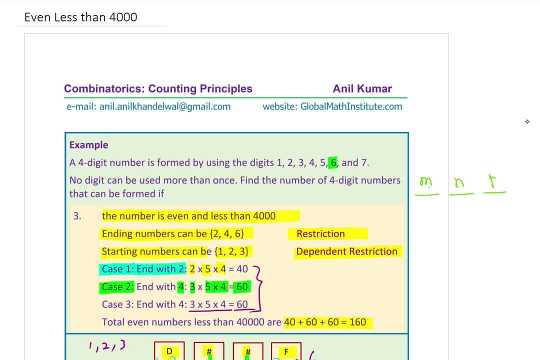 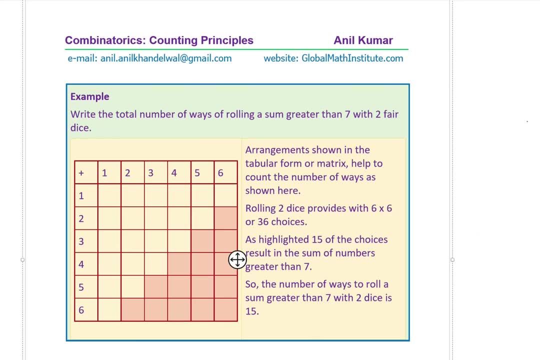 Let's say, if this option is m, this is n and this is p, then the answer is m times n times p. Is that clear to you? Okay, So that is how we are going to do it. Now here is another type of counting which is very popular. 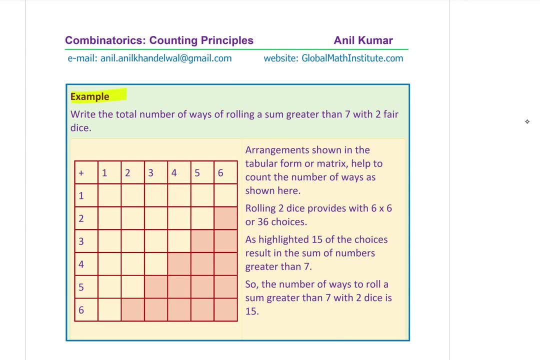 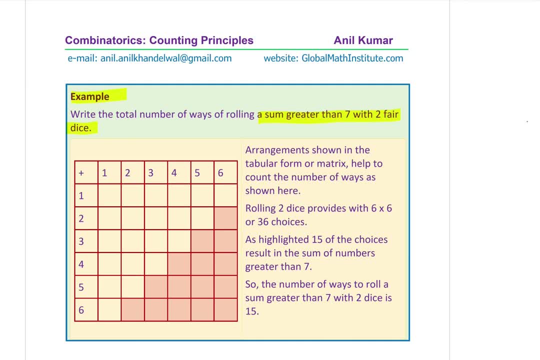 2: fair dice. That means you know, a dice has 6 faces, correct? So those 6 faces have 6 numbers on them And those numbers is what we are talking about, correct? So that is our dice And on this dice we have numbers mentioned, correct? 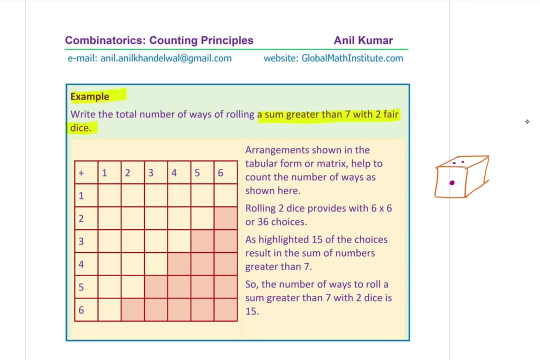 So let's say this is one number And then let's say this is like this. numbers are written: okay. so in this dice, when you throw, there are six options. these options are given to you in the form of rows and columns, as you can see here. okay, 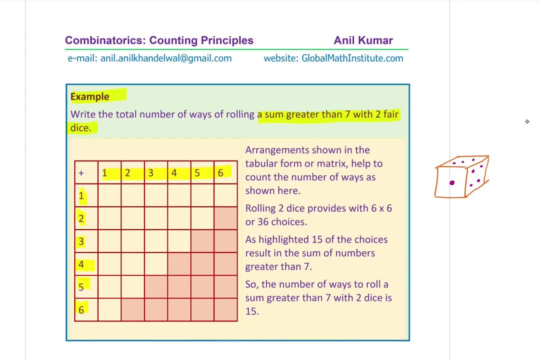 so two dice, so one die. we are saying die number one. so this is number one here and that is number two. so when you throw them you can add the numbers and the addition goes in this particular matrix form. is that clear to you? we're looking for a sum greater than seven, so this row here. 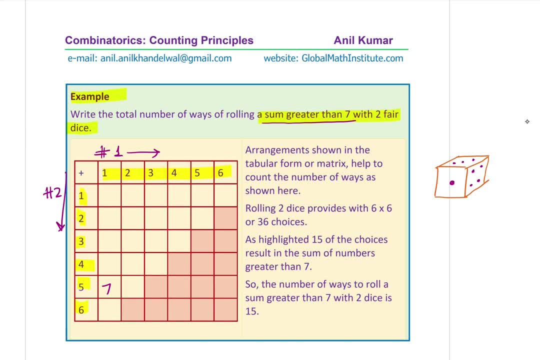 will give you seven, right? so seven- i mean six plus one- is seven. this is the row which will add to seven, correct? so if you add six and one, you get seven. so if you add six and one, you get seven. so if you add six and one, you get seven. so 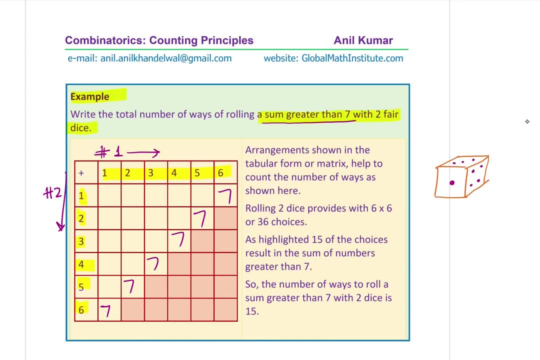 7, the row that diagonal, I should say 6 and 1,, 7, right, 2 and 5,, 7.. But if the number is below it, that is, 6 and 2, we get an addition here 8.. 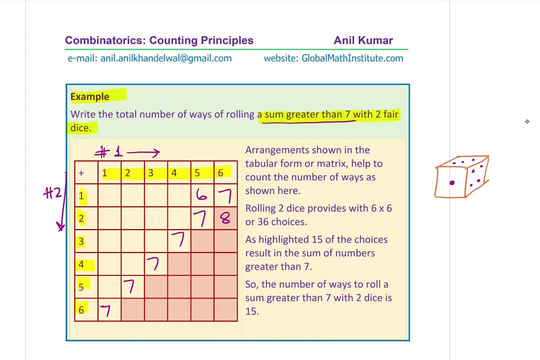 And if it is above it, we have a smaller number. Do you see that? So all these are the cells in which the addition will be greater than 7. We can just count them, And once you count, you see that there are 15 of these. 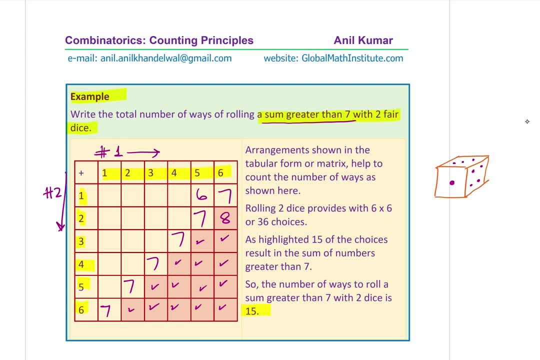 And therefore there are 15 ways of getting more than a sum of 7 when 2 dice are thrown. There are 36 in all choices right 6 times 6.. So there are 36 choices, out of which 15.. 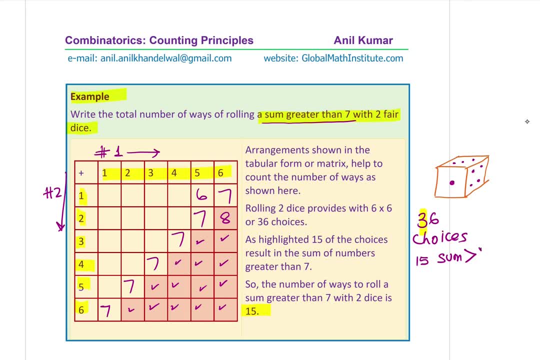 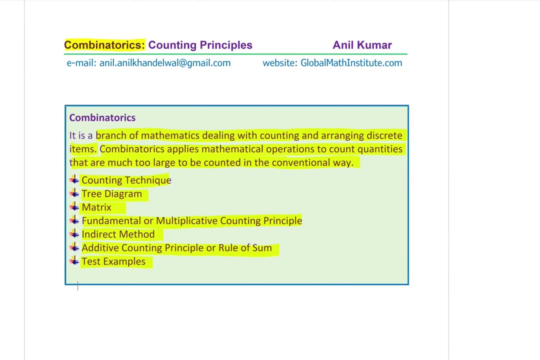 Is with sum greater than 7.. Is that clear to you, right? So that is how you could easily sketch and get your answer. So what we discussed here are different ways of counting, And that is combinatorics. Now, in combinatorics, the numbers could be very large, as we saw. 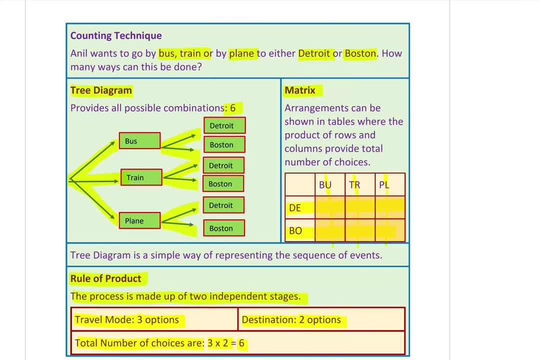 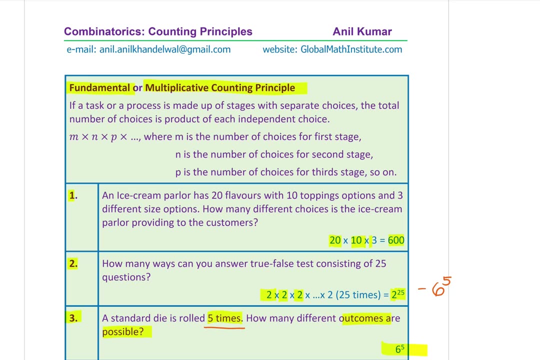 And these simple methods are effective for smaller numbers, especially the tree diagrams and the matrix. However, we could use the counting principles. the one which we decide on is the multiplicative counting principle. If we have independent cases and they are done in a sequence, then each option can be multiplied. 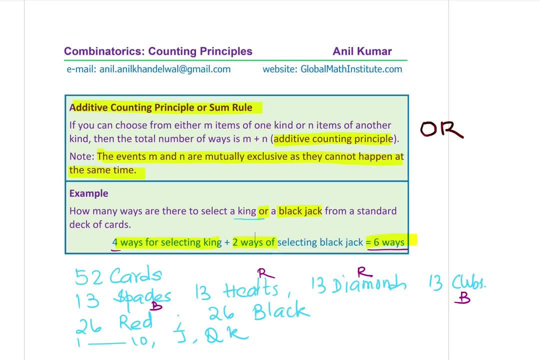 And the other one was if we have mutually exclusive, no overlapping, independent cases. in that case we could add the options And we also saw that sometimes we may have to use more than one alternative right. So these are different ways of working with counting and arranging.